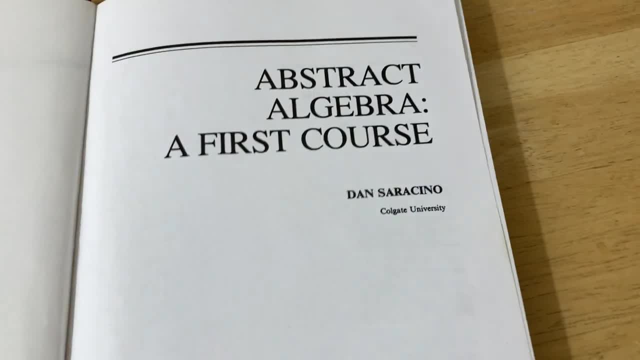 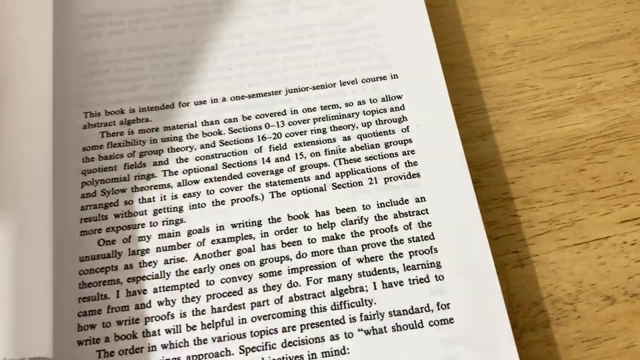 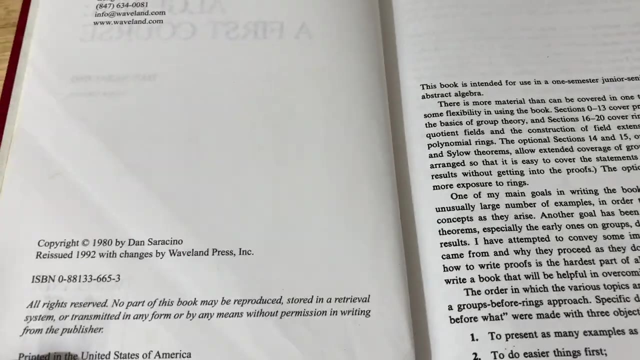 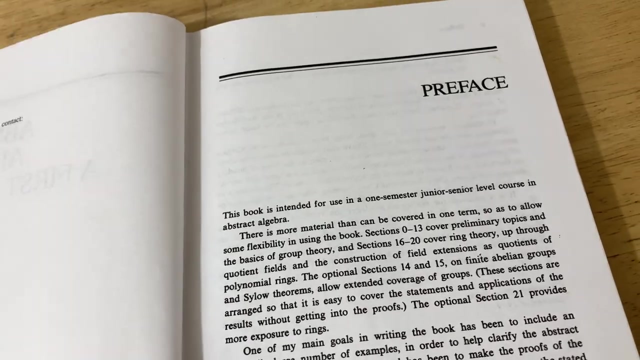 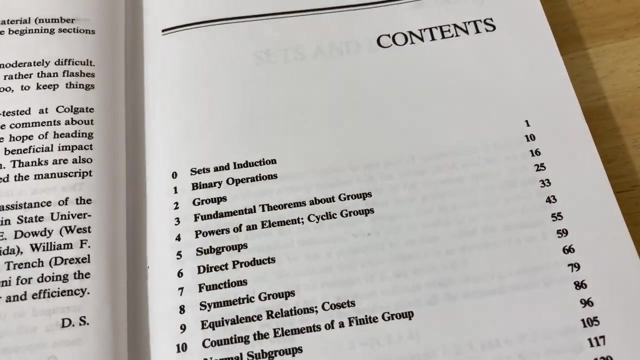 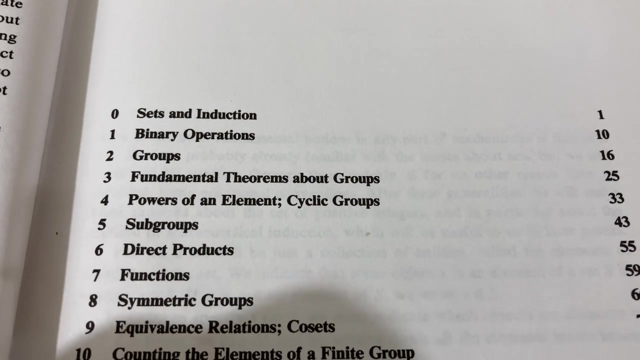 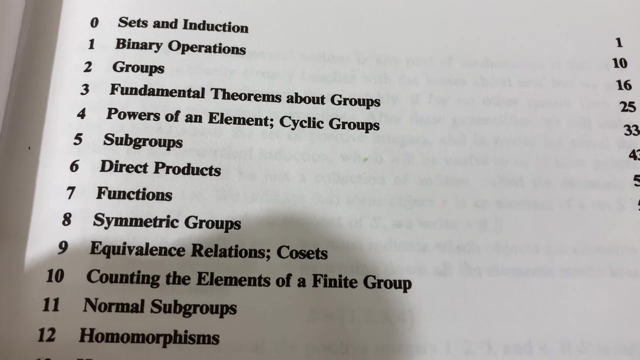 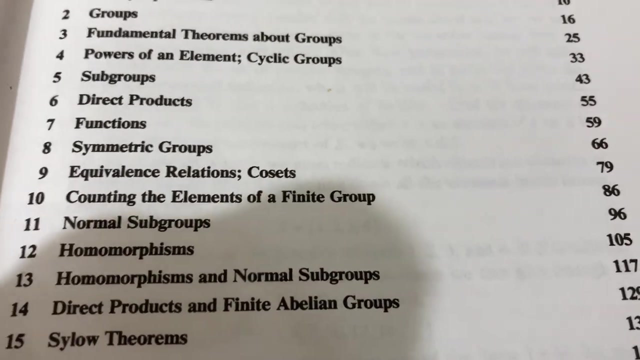 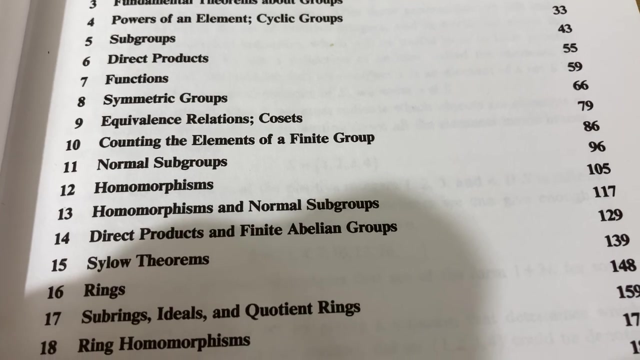 So let's just go ahead and open it up. I'm going to show you the inside. Abstract Algebra, Dan Cerachino, Colgate University, Waveland Press, Inc. I actually, long ago, I taught a course with this book. It was kind of like a little independent study with just a couple students and we went through a decent amount of the book and these were students that they didn't really have like a proof writing background so i had to teach them how to write proofs and some of them were really awesome so here's the contents so you can see starts with sets and induction binary operations groups fundamental theorem about groups powers of an element cyclic groups subgroups direct products functions symmetric groups equivalence relations and cosets counting the elements of the finite group so it's like lagrange's theorem normal subgroups homomorphisms homomorphisms and normal subgroups direct products and finite abelian groups the silo theorems rings sub rings ideals and quotient 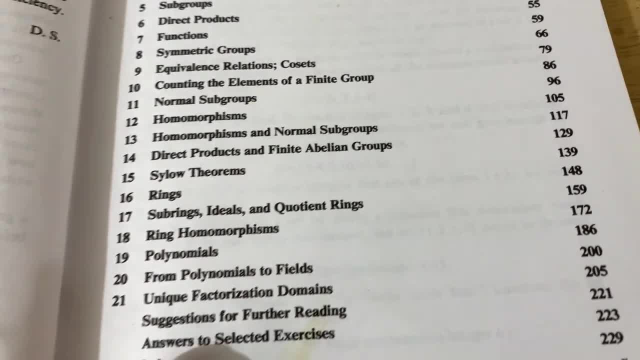 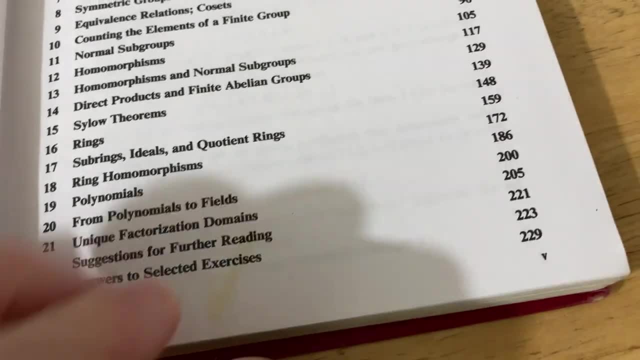 rings ring homomorphisms polynomials and then from polynomials to fields and then ufds which are unique factorization domains answers to selected exercises so it does have some 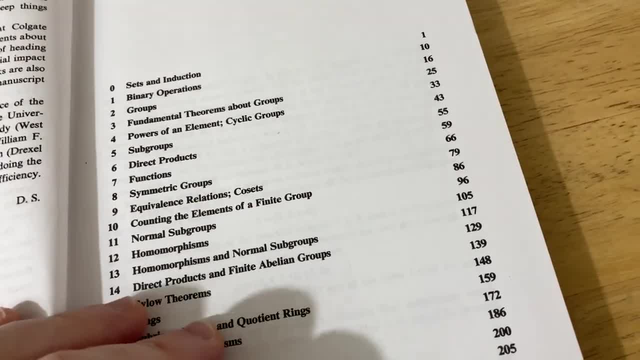 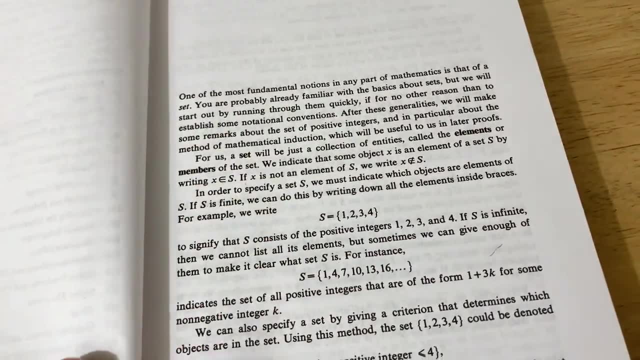 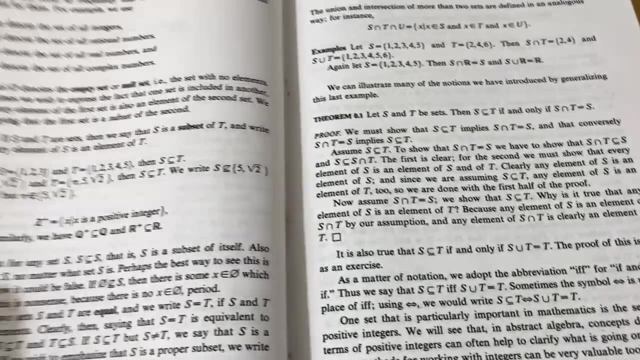 answers to some of the problems but i would i would say it's not significant you're really not going to get that much in terms of answers so it starts off with sets and induction and it has like this introductory section on induction which you could read and you could learn from if you didn't know about sets and induction i have pretty much read i think this entire book i've actually read 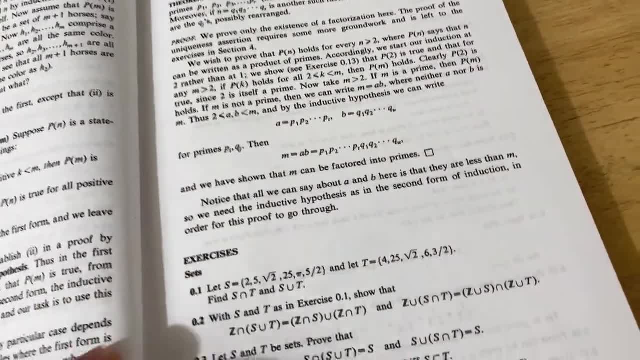 the entire thing and i've done a lot of the problems apparently i didn't do these though usually i would 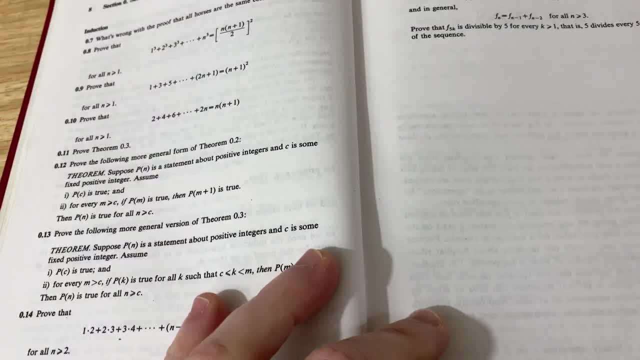 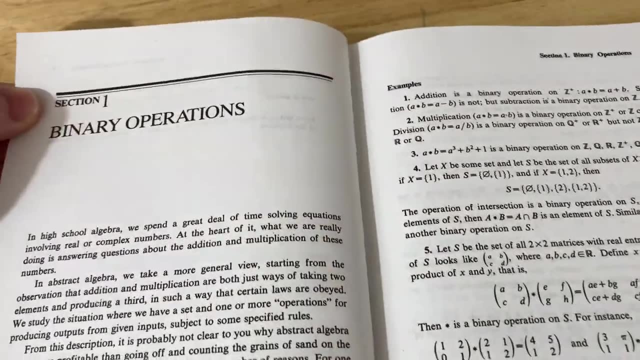 or scratch them out but i kind of feel like i have done these so maybe i just didn't want to write in the book because you know i've worked through uh pretty much the entire book section one's on binary operations so i know i've done a bunch of the problems here and again i just for 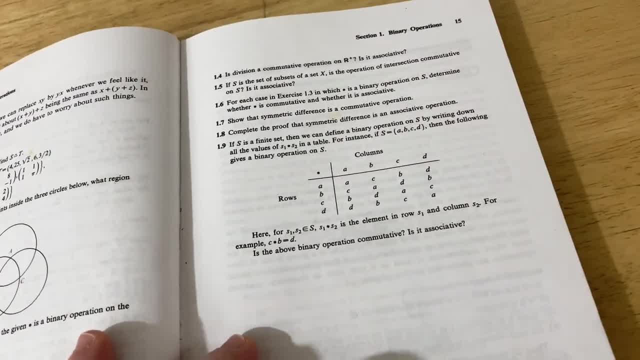 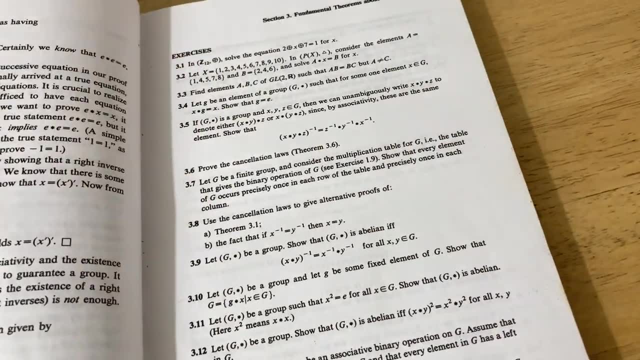 some reason i didn't write in the book which i probably wouldn't today i've got a pencil here and i'm not going to write in this book so yeah um so the pros of this book are that uh it's very 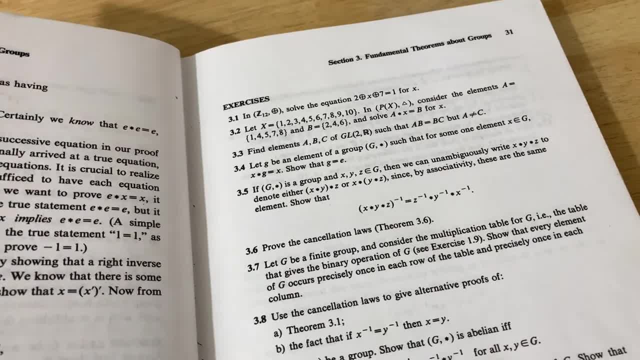 easy to read it's very well written and it has exercises that are appropriate for the level of 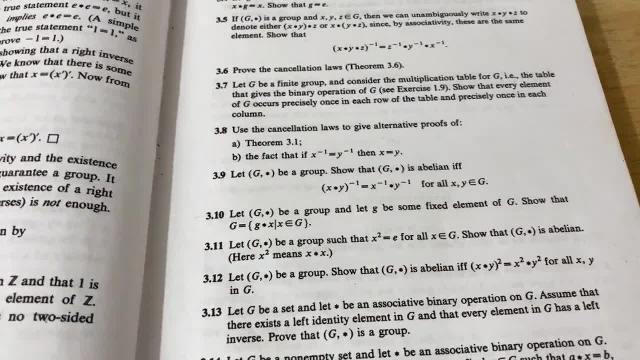 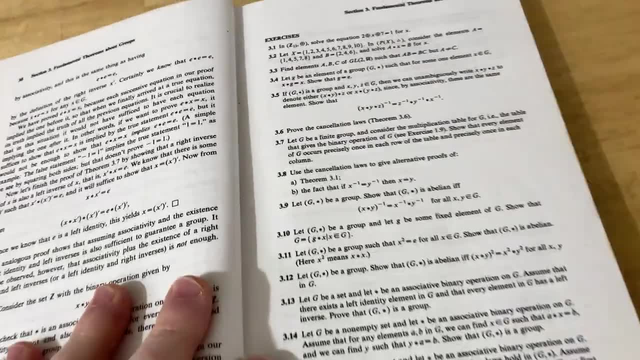 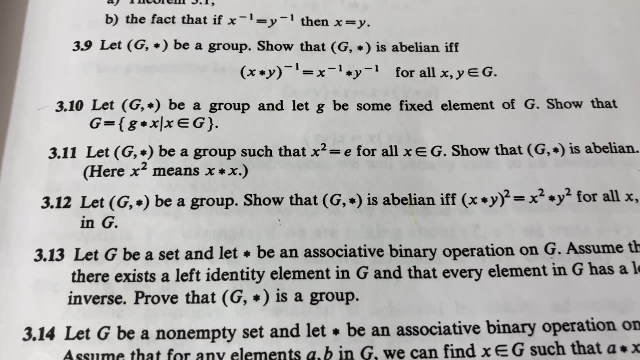 reading also a lot of the problems are very standard so you'll find them in other books and if you're taking a class in college by having this book even if you already have a book you'll get you'll gain access to extra exercises which might end up being test questions for example here's some very popular problems look at number 11 let g be a group such that x squared equals e for all x and g show that g is a beeline for x squared equals e for all x and g show that g is a 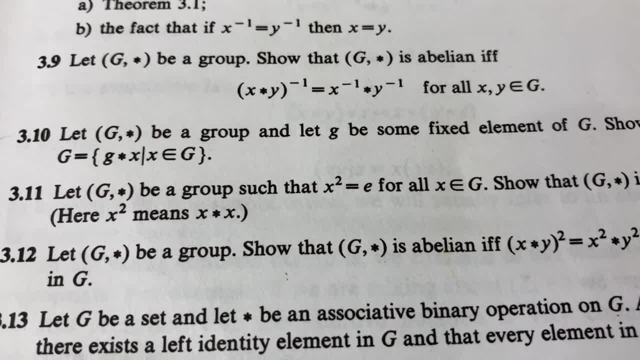 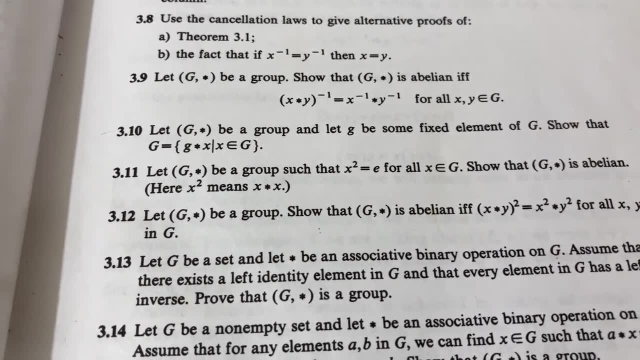 so if you think about that statement if you know any group theory uh basically saying x times x equals e that means that every element uh in this group is its own inverse uh which is pretty cool 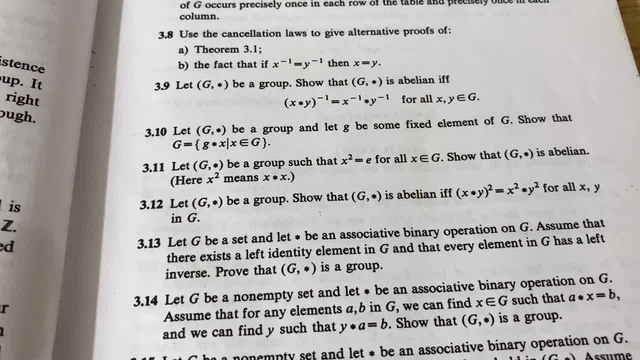 and when that happens uh the group is a beeline so yeah this one's a little bit harder 14 is a 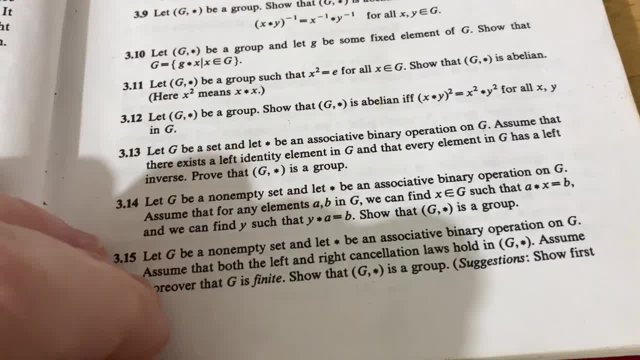 little bit harder and so is 15 15 is a little bit harder as well yeah pretty cool and then four goes on to cyclic groups 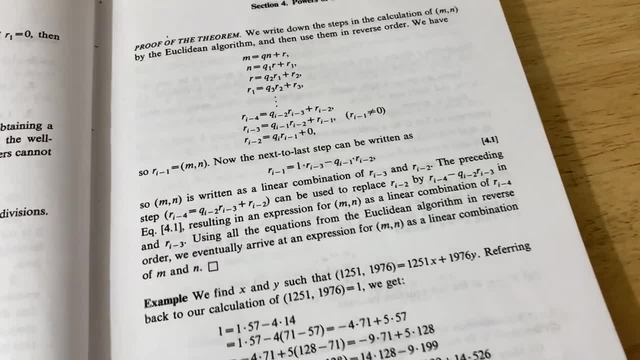 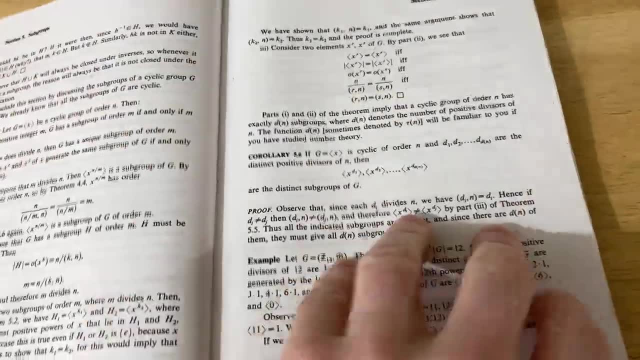 does pretty good here one of the things that is lacking in this book is content so for example if you want to learn like feel theory or galois theory let's go to the back of the book i mean 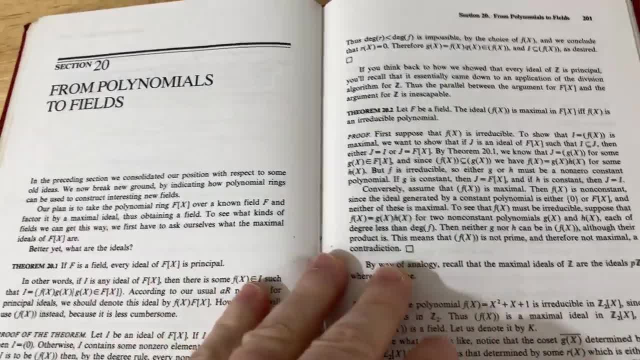 it does do some stuff right it talks about polynomials but this is section 20 and so now it talks about ufds 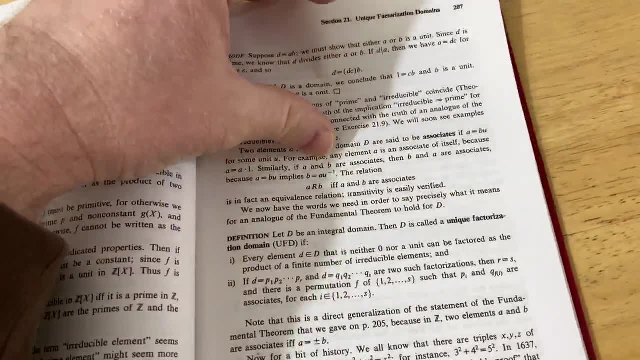 i actually read these sections uh via self-study when i was a graduate student because when i was 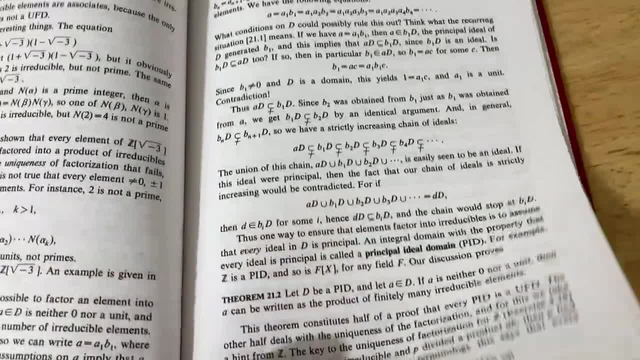 an undergrad we didn't cover all of these sections talks about pids okay and it eventually 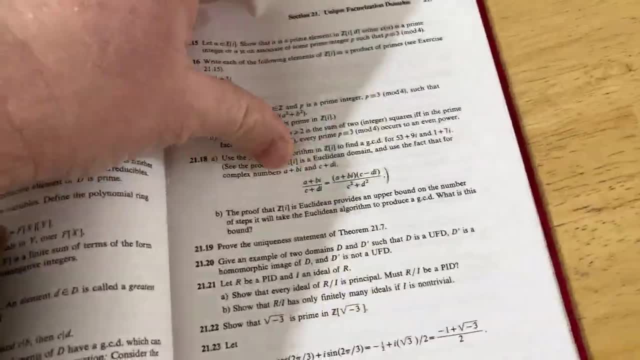 ends i think this might be the last section let's see that's it right suggestions for further 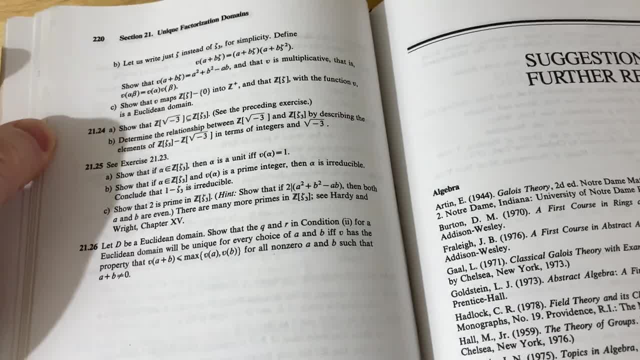 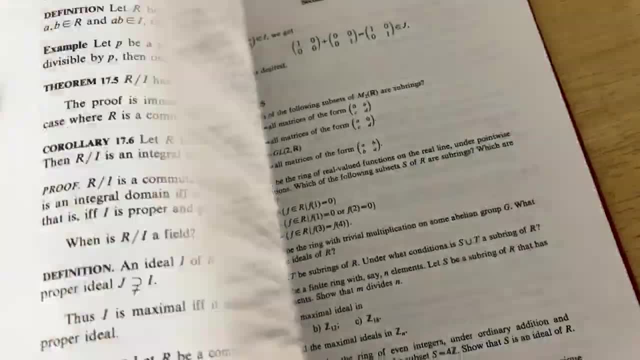 reading so that's it so the book ends and that's honestly one of the the worst things about the book another con is sometimes um the proofs in the book i mean they all well written but 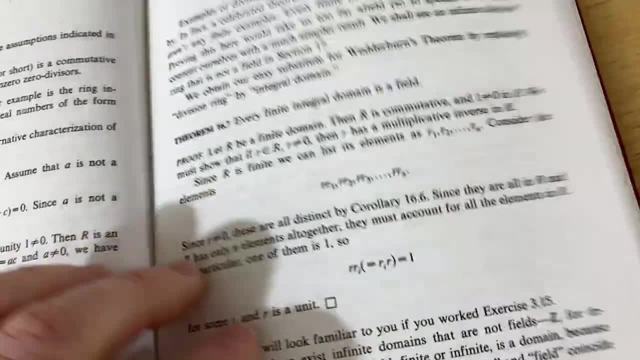 um the best proofs are the ones you write so for example here's a proof where they show every integral domain as a field um i actually have a youtube 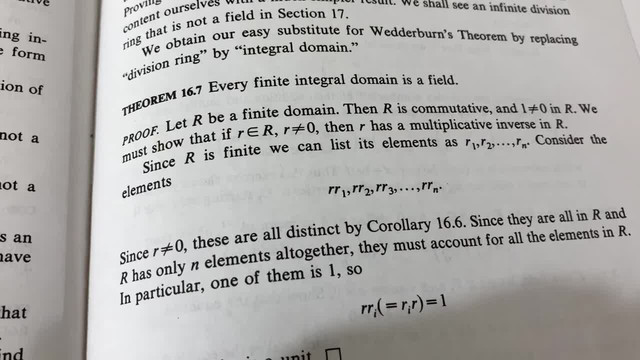 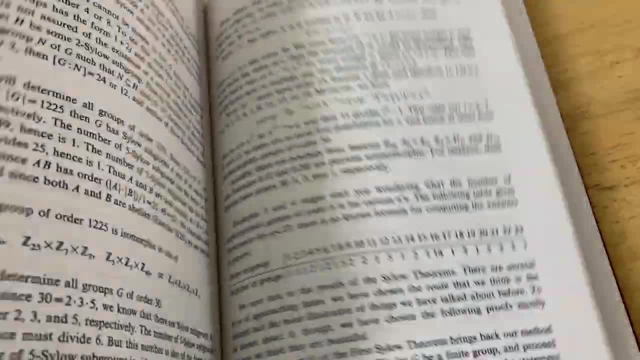 video of this proof that i wrote so um it always makes more sense when you write it so good book i think it's worth buying if you are trying to learn abstract algebra 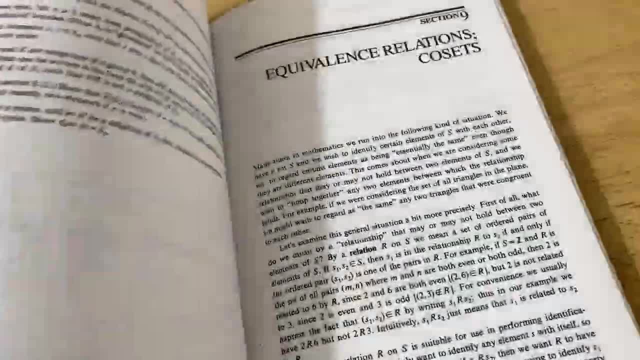 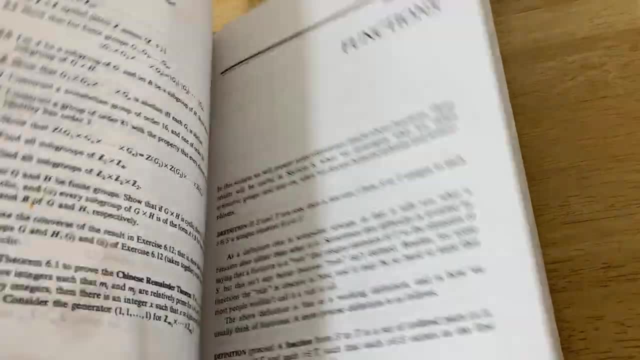 if you're a book collector yeah definitely worth picking up if you can find a copy at a reasonable price i don't think this book is super inexpensive anymore when i 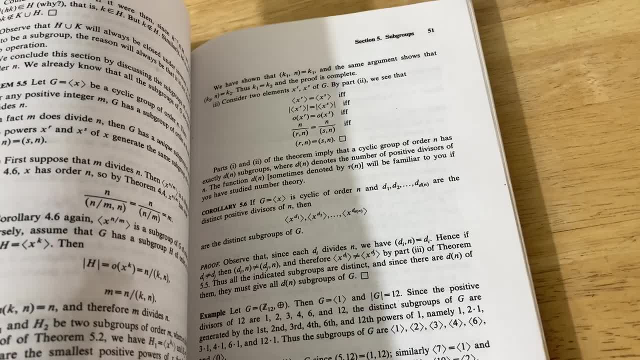 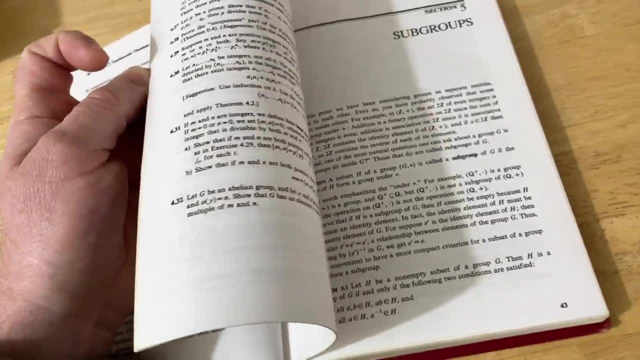 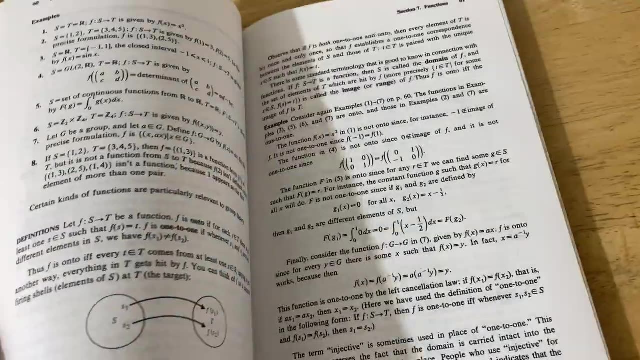 bought my copy several years ago. I paid like, not so, well, I think I paid, I think I bought it new. And then I think copies after that, used copies were about 10 bucks a piece or so, or maybe less. But I think the price has gone up since then, you know, inflation and all that stuff. But 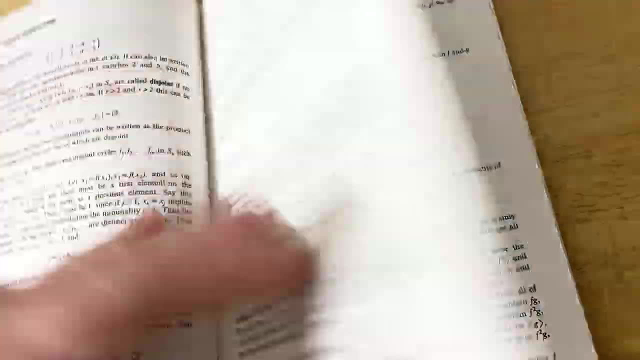 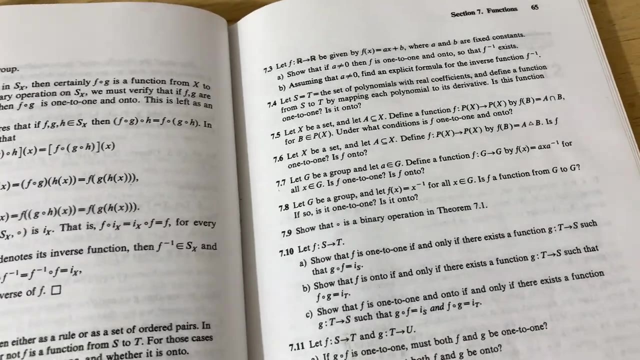 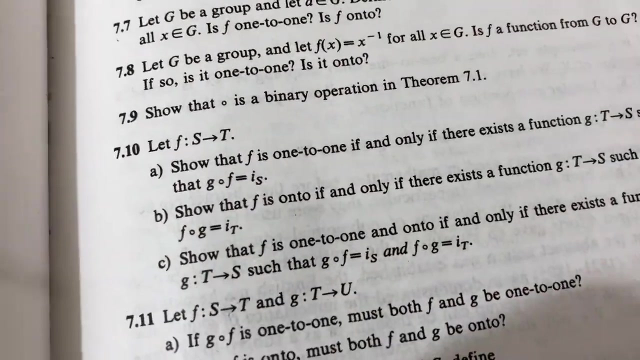 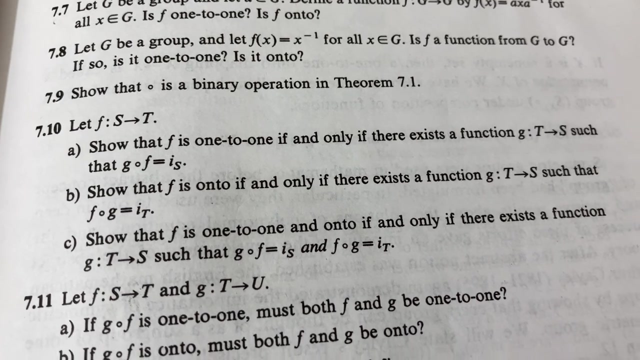 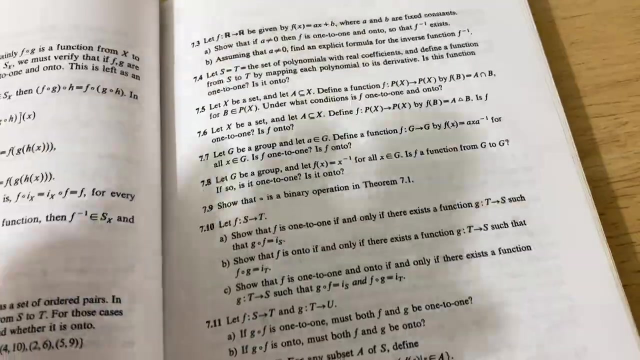 yeah, pretty good book. It's got a nice extra, nice sections on functions that appears before symmetric groups. So yeah, these are things that you would see maybe in a proofwriting class or in a discrete math class, you would prove a lot of these things. For example, here, number 10, show that f is one-to-one if and only if there exists a function g such that gof equals the identity on s. And then here you have some other things that you would prove, perhaps in a proofwriting class. So very nice book. I recommend it. Good for beginners, a lot of people. But yeah. 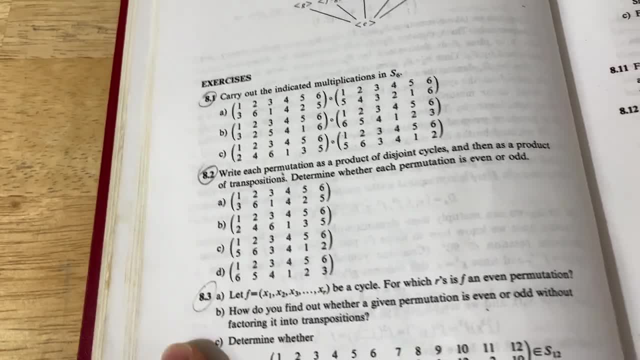 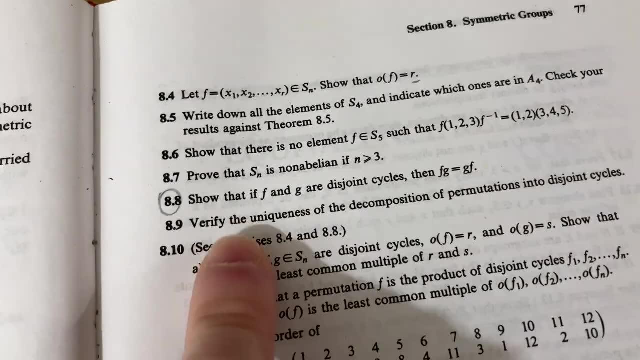 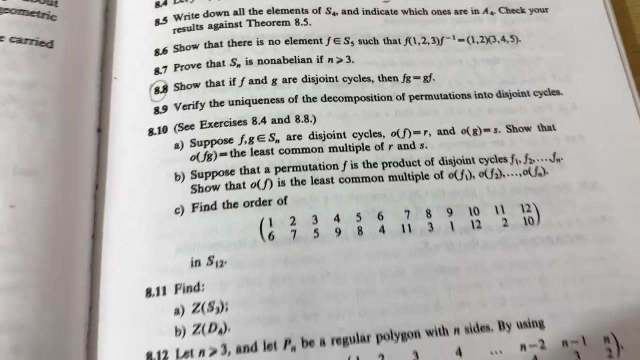 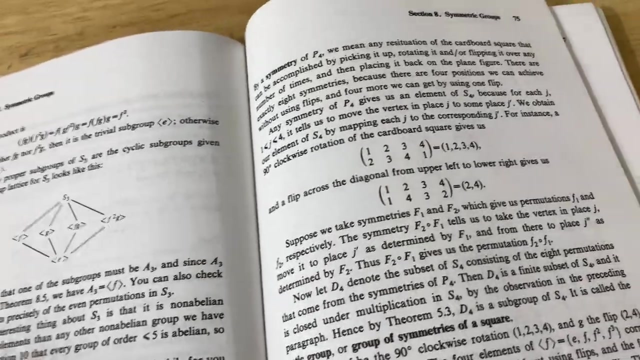 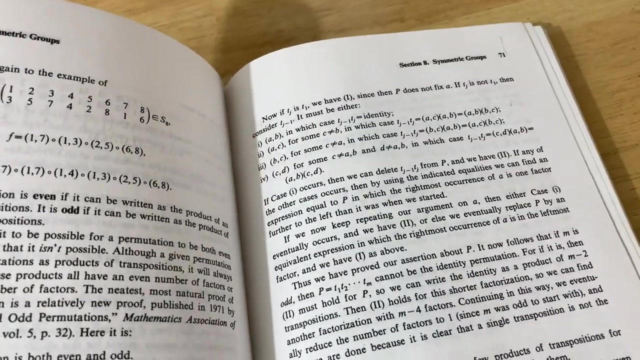 look, look at this, I've circled some stuff here. It's funny because, you know, I've done most of the exercises in this book, but I decided to circle these and I didn't circle the other ones. I also did this one here, show that F and G are just joint cycles. If there are just joint cycles, then FG equals GF. Cool. Yeah, this is on the section on symmetric groups, which it's a tough section for people to learn. It takes some time to get used to the proofs in dealing with symmetric groups. And the Cycle Multiplication is actually easy once you learn how to do it. This book does actually have good examples of Cycle Multiplication, I